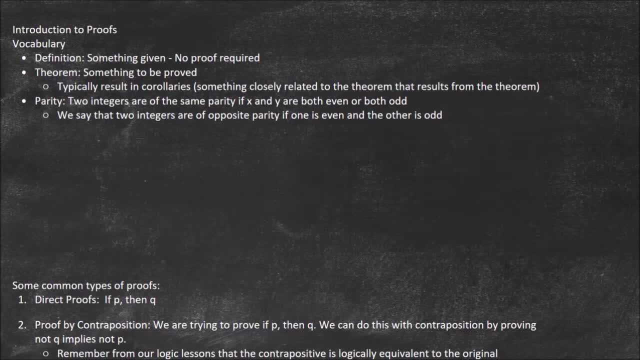 what you're trying to work for, And it typically results in corollaries, which are basically things that result from the theorem, So really closely related to the theorem that you've proven, but not the exact thing. And then another important term is parity, And this means that two integers are of the same parity. 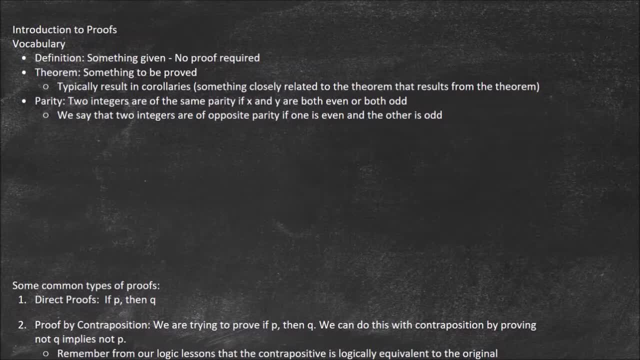 if x and y are both even or they're both odd. So we say that integers are of opposite parity, of course, if one is even and one is odd. So just know that term, because that shows up a lot in proofs. They might say: well, if they have the same parity, is this even? 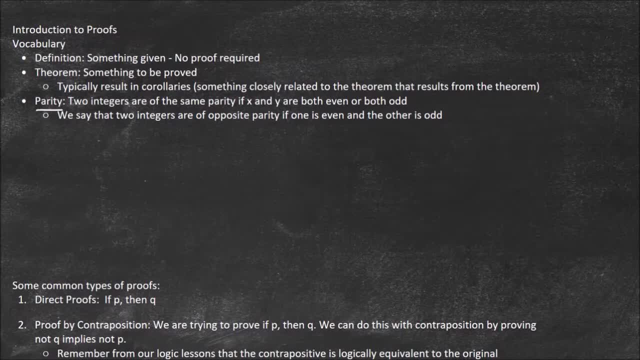 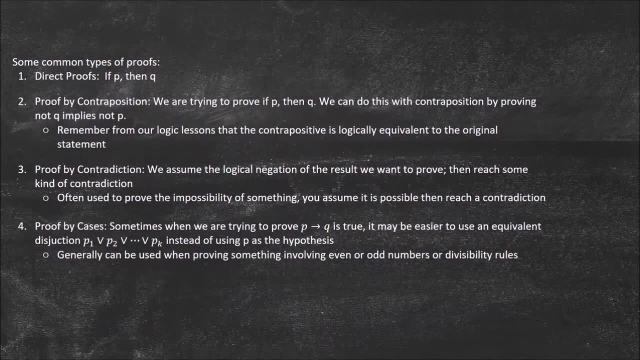 or odd. So you need to be able to tell, well, what does it mean? that they have the same parity And that just means that they have the same even or odd status. So so, common types of proofs. So these are the ones that I'm sure you might have done. 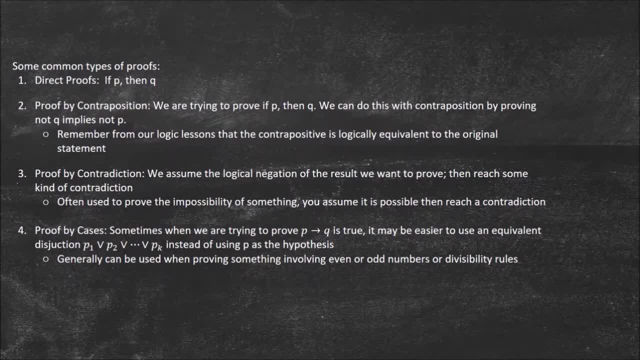 some of these before, but just just the basics here. So direct proofs: if P, then Q. that's the most basic thing. you directly try to show that well, if P is true, Q must be true. The thing is with direct proofs is you can't do them all the time. They're going to throw. 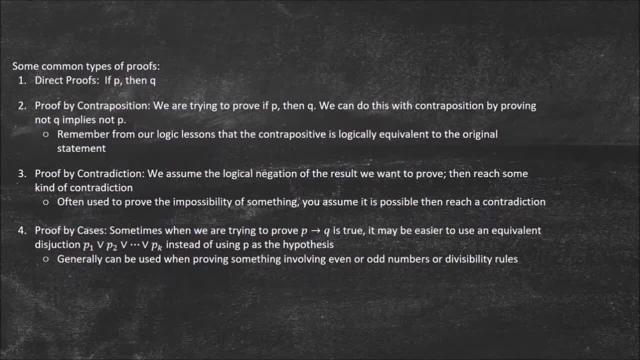 tricks in there to just make it to where you can't just directly plug in whatever P is to arrive at Q. Next we have proof by contraposition. This is a common one where if we're trying to prove P and then Q, we can do this with contraposition. by proving not, Q implies not. 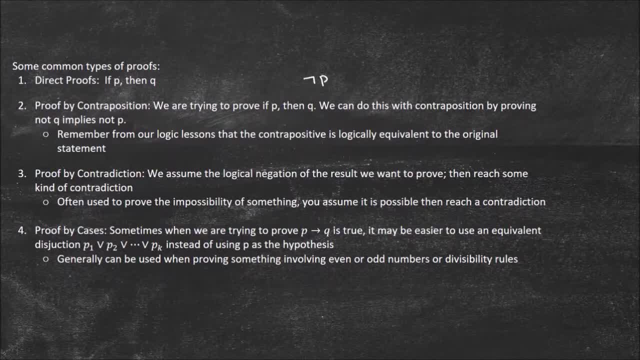 P. So remember, in our logic section we did not: P implies not Q. That's equivalent to P implies Q. They're logically equivalent. If you want to do a truth table, you could do that and you'd see that they're the same. So that's another way to do a proof We can. 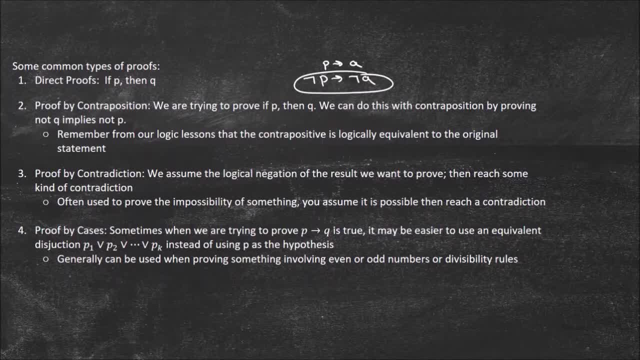 just do the contraposition here instead of um. actually wait, this should be not. Q implies not P, Misspoke there. So not Q implies not P. So that's the contraposition. So sometimes that's easier. Sometimes it's easier to say: 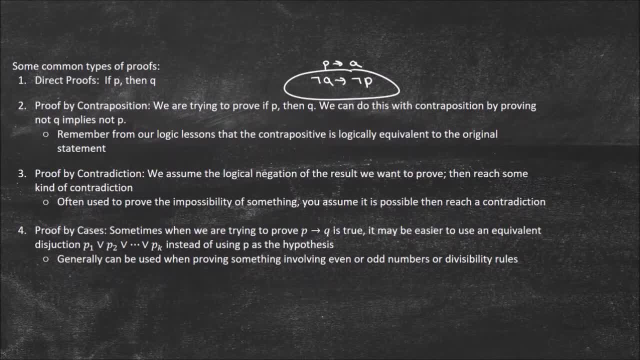 well, what if the conclusion is just false? Can I easily show that the hypothesis is false? And that can definitely happen sometimes. And if you wanted to do a statement, a truth table, you could, and I almost recommend it, just to make sure you feel good about contraposition. 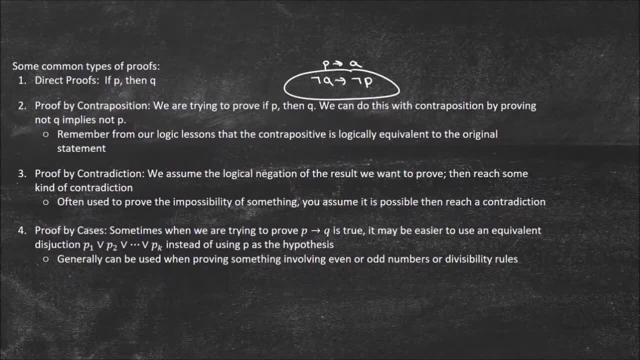 So next we have proof by contradiction. Here we assume the logical negation of the result. Then we reach some kind of contradiction, So we assume the opposite of what we want to prove. So we kind of assume not Q, and then we show why P just can't happen. So it's used to show. 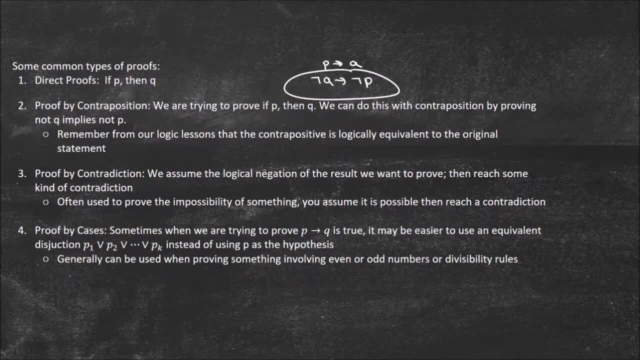 the impossibility of something, You assume it is possible and then you reach some contradiction. So you use this for things like proving rational and irrational numbers. This um, so that can be a harder one. I think proof by contradiction is one of the tougher sections of this um. 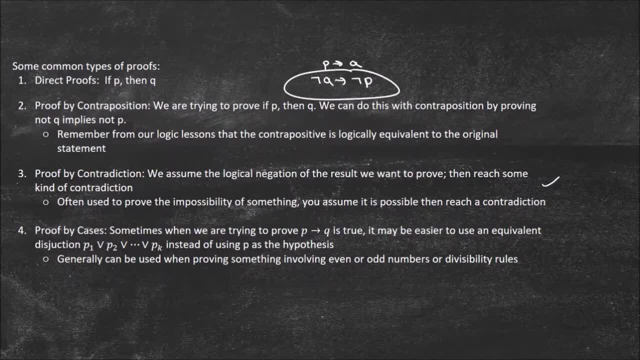 unit. but we have some examples and you'll feel good about it by the end. And next we have proof by cases. So sometimes, when we're trying to prove directly, P implies Q. it can be either P1 or P2 or all the way to PK. instead of using P, And this is common when you kind 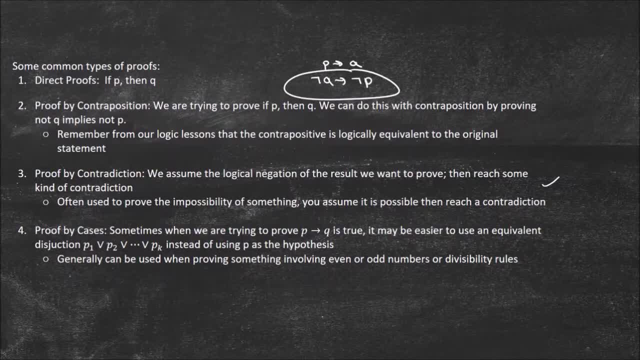 of have like: if N is an integer, then this happens. Well, there's two cases where N is an integer, It can be an even integer or an odd integer, right? So it's easier to show that well, when it's even, this happens. When it's odd, this happens, Then it must. 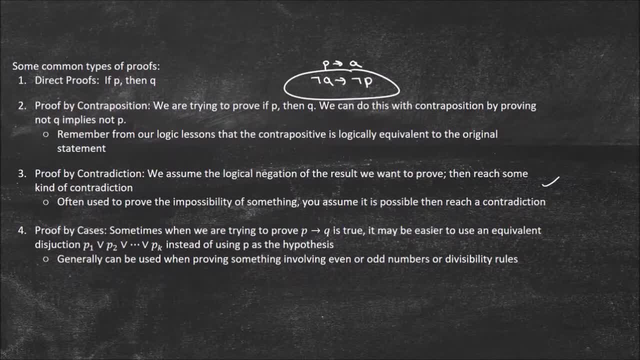 happen all the time. So that's a common thing And that it's this is a good one to know, proof by cases. Most teachers, most teachers, cover it, Some don't. And the ones that are don't, I think really are doing a disservice- disservice because they can really make you. 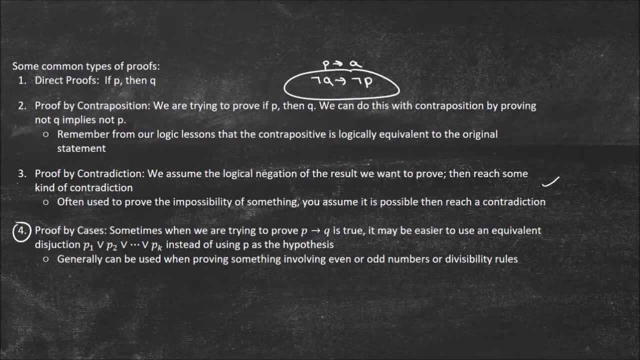 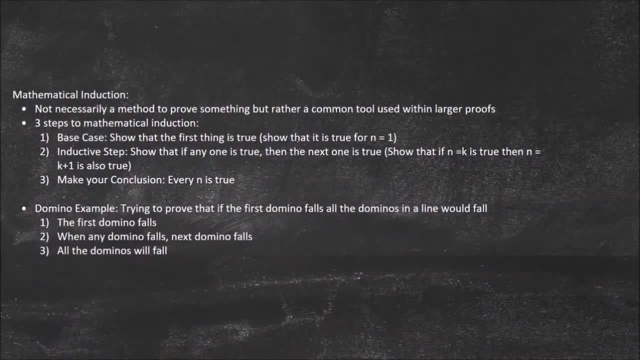 do some of these a lot quicker and they can make more sense. So basically this: you'll see some examples later on, but this is a good way to do some proofs. And then we also are going to cover mathematical induction. This is kind of a proof method. It's kind 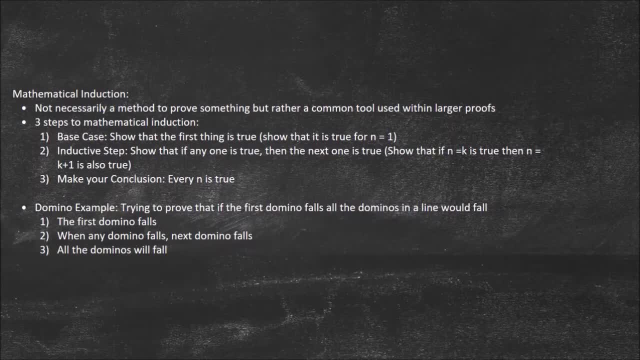 of something used within proofs a lot, And this is a common tool for um just showing that well, if if this happens, then this has to happen for all cases. So what you do is you're going to show that the first thing is true If it works, for n equals one, and 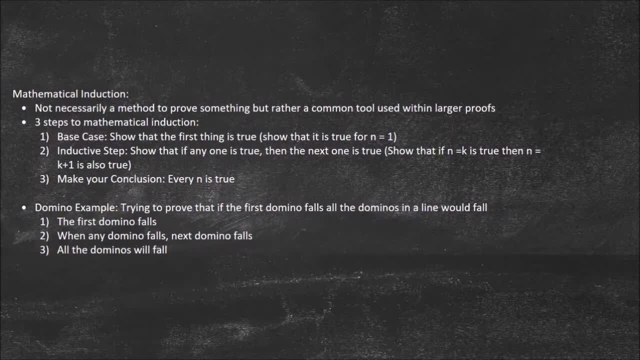 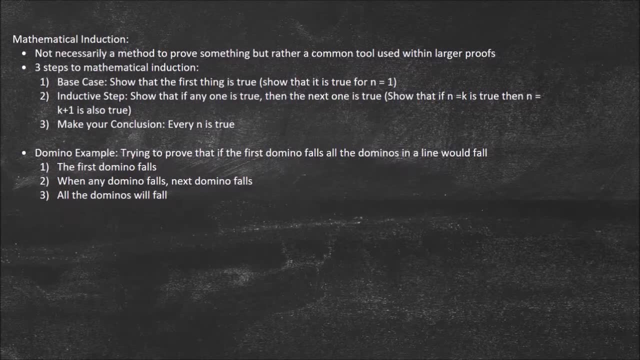 then I can show that it works for the- for n equals k plus one- then I can show that it works for everything. So the logic, we'll get into this much more in the actual video, but the logic is with dominoes. So if the first domino falls and then I can say, well, 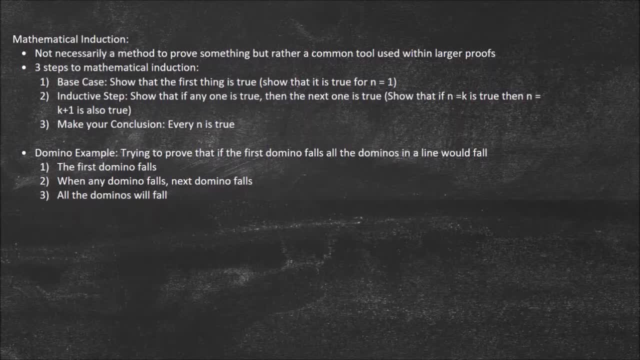 the second step would be: when any domino falls, the next domino falls. So notice that I've said the first domino fell And I say that when any domino falls, the next domino falls. Well, if the first domino fell and the when any domino falls, the next domino falls Well. 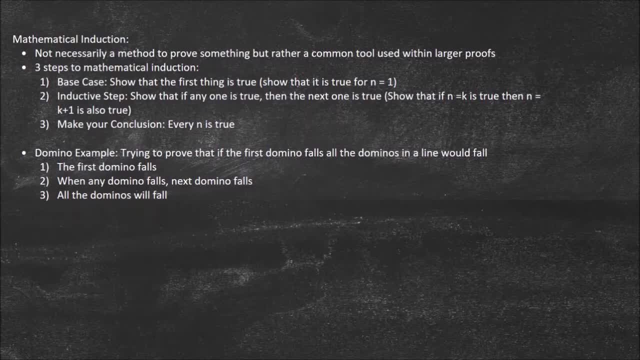 if the first domino fell and the when any domino falls, the next domino falls. So notice that when any domino falls, the next domino falls. I know the second one fell, which implies the third one fell, And you can go step by step all the way to assume all the. 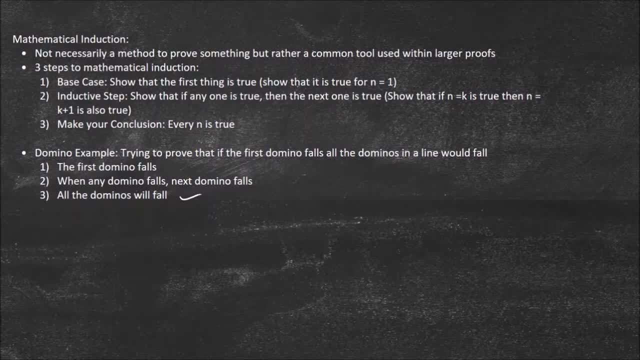 dominoes will fall. So that's kind of the logic of mathematical induction. Hopefully that makes sense. We'll get into a lot more with that And mathematical induction can definitely be one of the harder parts of this course, So definitely pay attention to that. 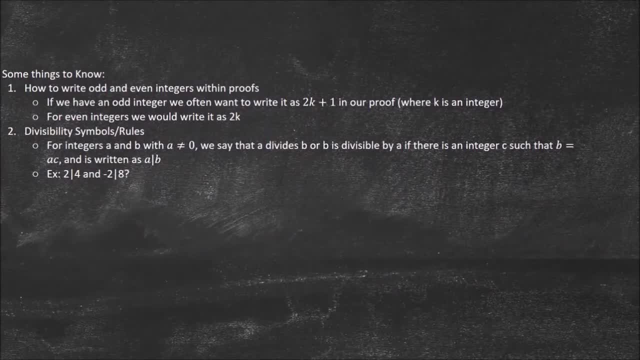 video. Then, lastly, just some things to know. So how to write odd and even integers within proofs. You may know this, but if we have an odd integer, we want to write it as two k plus one, Where k is an element of z, which means k is an integer. Just the common way to write. 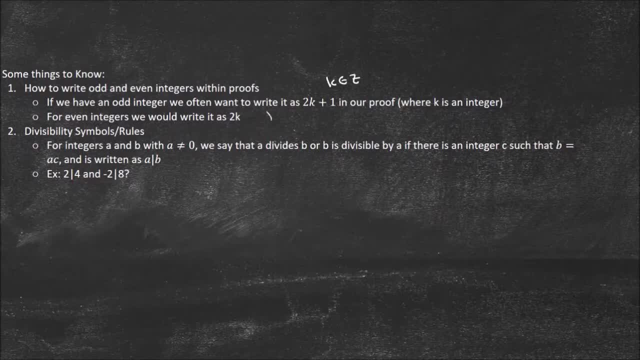 the odd numbers. Then for evens we just write it as two k, where k is an element of z again, And the reason we do that is just because it's the simplest way to write them And then we can from there we can plug them into all kinds of formulas and things like that. 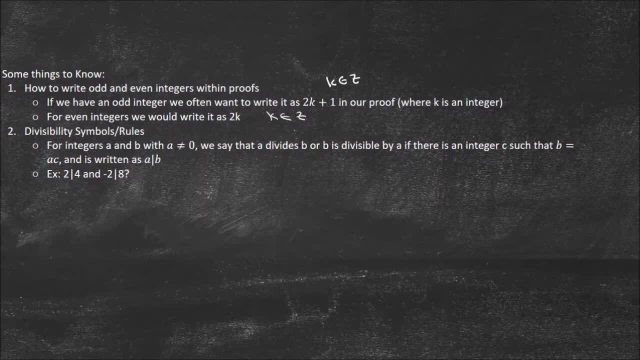 You're going to see that all the time. Then the divisibility symbols and rules. This one's a little less intuitive, but so for any integers a and b, with a not equal to zero, we say that a divides b Or b is divisible by a. if there's an integer c, such that b equals ac. So that seems really. 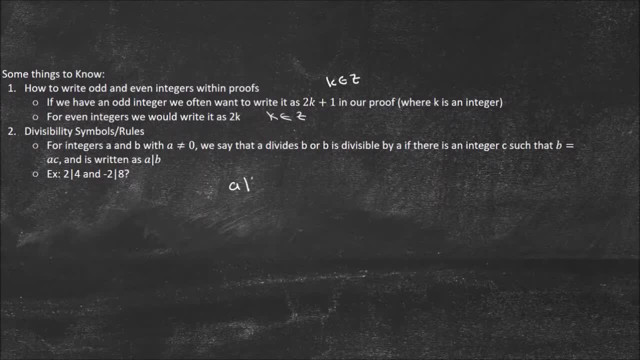 confusing, but basically it's written as ab. So a divides b. That's what you need to read this as A divides b. You will sometimes see this in proofs, So let's look at an example. So does two divide four? Yes, it does right, Because four divided by two is two Does negative. 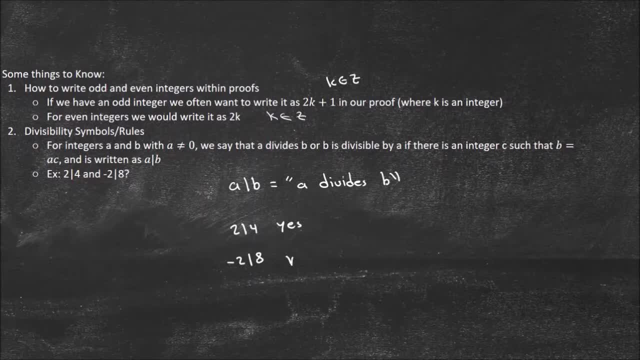 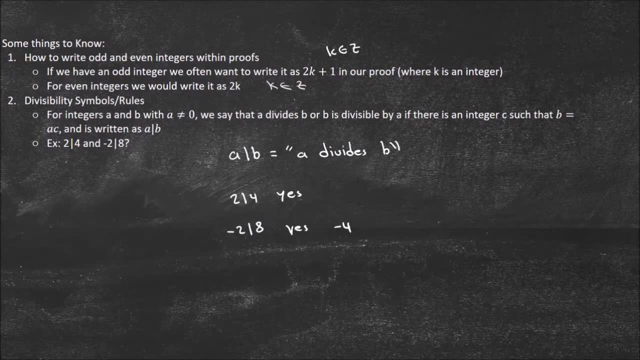 two divide eight: Yeah, it does right, And the answer would be negative four. So I can do eight divided by negative two. An example of when it wouldn't work would be: does three divide four? No, it doesn't. It equals a decimal. Yeah, So it only works if there's an integer c, such that b equals ac.